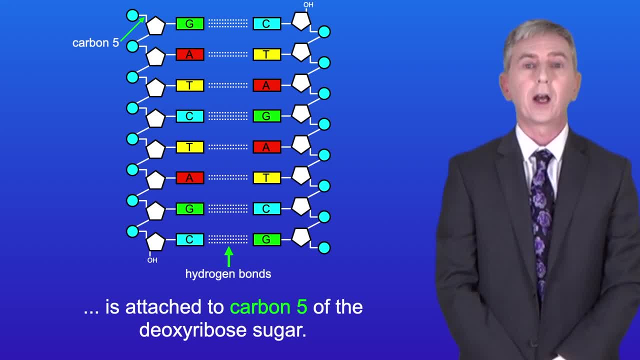 the top phosphate group is attached to carbon-5 of the deoxyribose sugar and at the bottom we've got the hydroxyl group attached to carbon-3.. On the right-hand side we have the carbon-3 hydroxyl at. 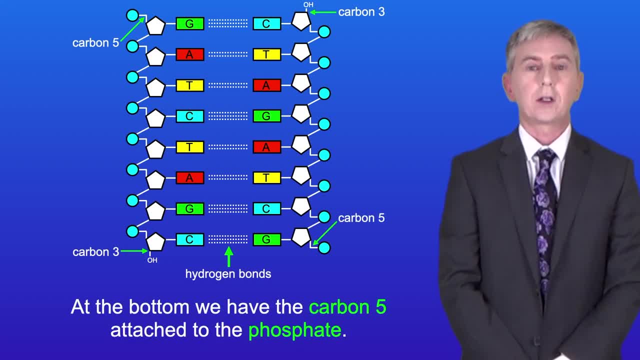 the top and at the bottom we have the carbon-5 attached to the phosphate. Secondly, the different base pairs form a different number of hydrogen bonds. Guanine and cytosine form three hydrogen bonds, whereas adenine and thymine form two hydrogen bonds. 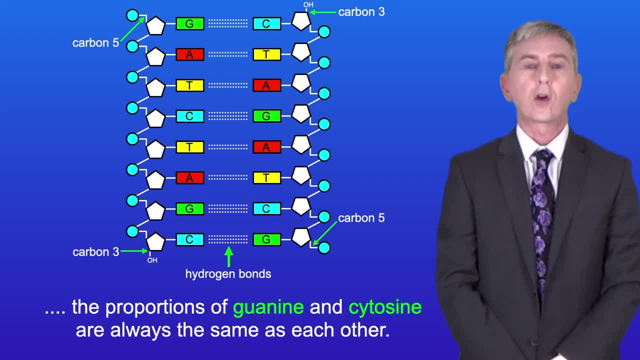 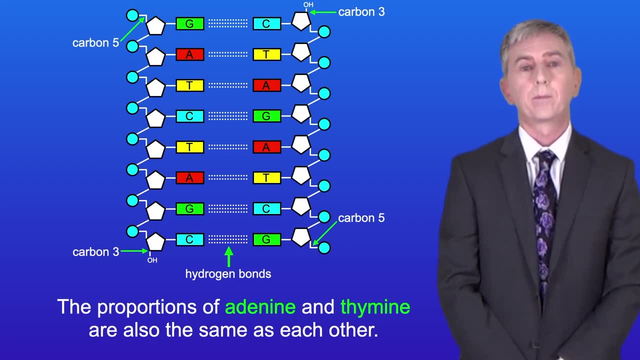 Now, because of complementary base pairing, the proportions of guanine and cytosine are always the same as each other, and the proportions of adenine and thymine are also the same as each other. This means that we can calculate the proportions of the different nucleotides. 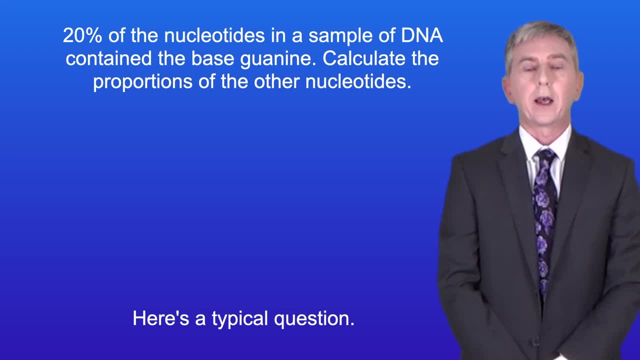 Here's a typical question: 20% of the nucleotides in a sample of DNA contain the base guanine. Calculate the proportions of the other nucleotides? Well, if we know that 20% of the nucleotides contain guanine? 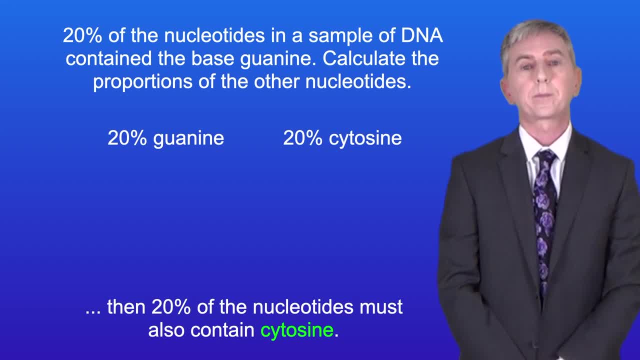 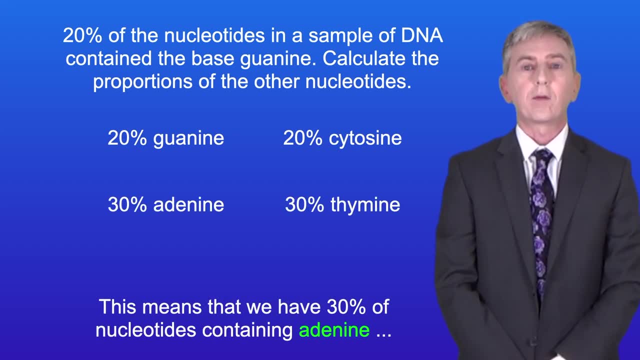 20% of the nucleotides must also contain cytosine. The remaining 60% of nucleotides must contain adenine and thymine. So this means that we've got 30% of nucleotides containing adenine and 30% containing thymine. 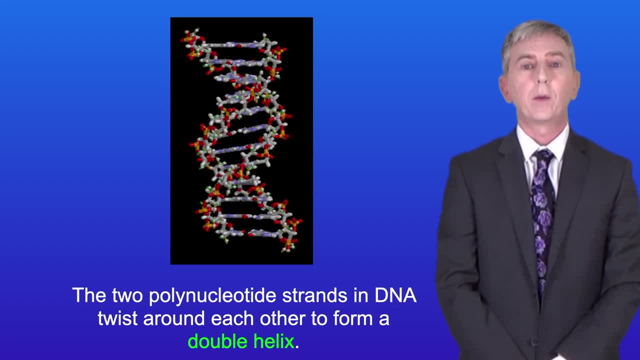 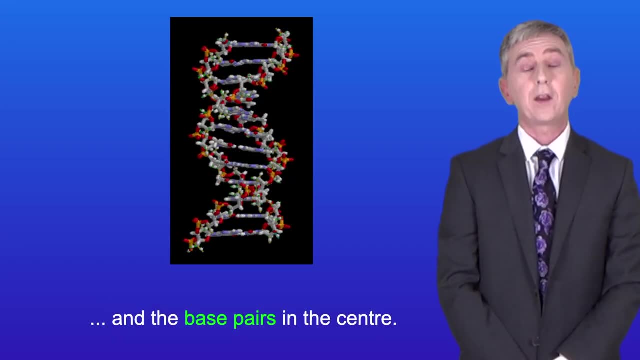 Now the two polynucleotide strands in DNA twist around each other to form a double helix and I'm showing you that here, So we can see the sugar phosphate backbones on the outside and the base pairs in the center Coming up. we look at the structure of RNA. 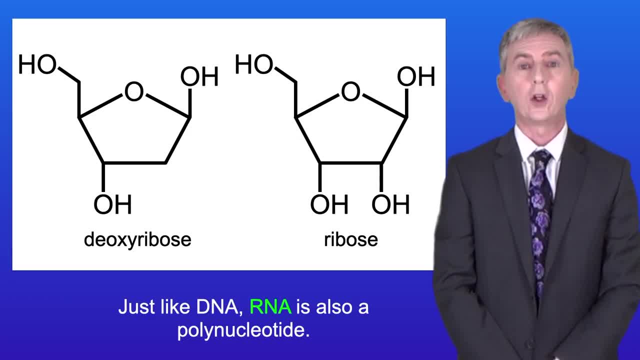 OK now, just like DNA, RNA is also a polynucleotide, but RNA is different from DNA in a number of key ways. We saw in the last video that RNA contains the pentose sugar ribose rather than deoxyribose, which is found in DNA. 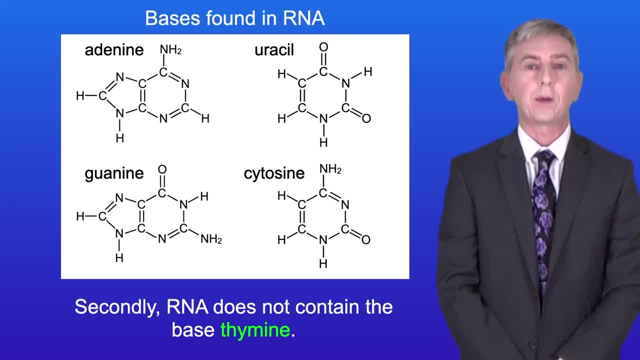 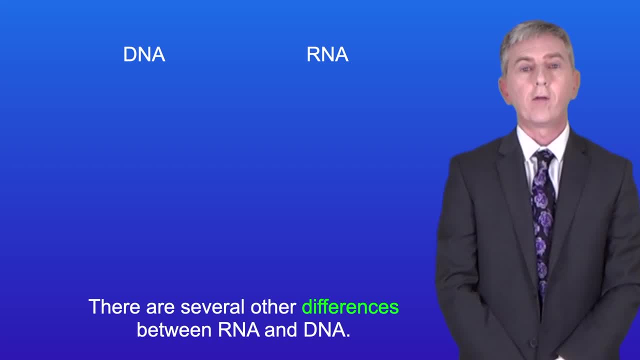 Secondly, RNA does not contain the base thymine. Instead of thymine, RNA contains the base uracil. Now, there are several reasons why RNA is different. several other differences between RNA and DNA. Firstly, DNA is found in chromosomes, in the